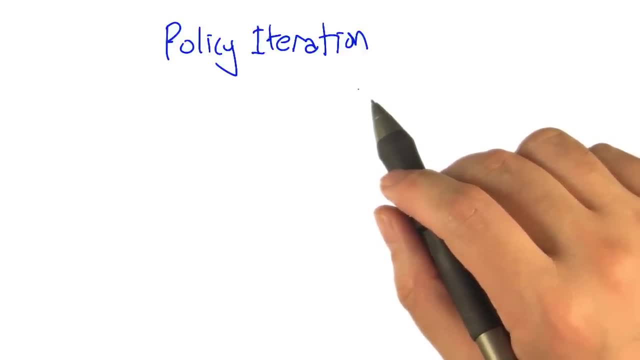 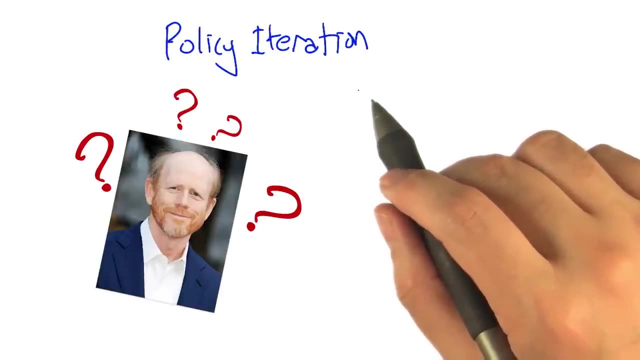 because it dates back to, you know, 1960 or thereabout. Dijkstra Dijkstra always has ideas before I do. Yeah, Dijkstra Dijkstra's pretty clever, but this was actually Ron Howard. You mean the Ron Howard, the, the rector. 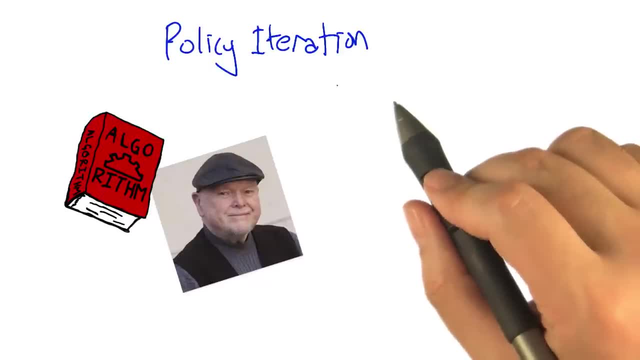 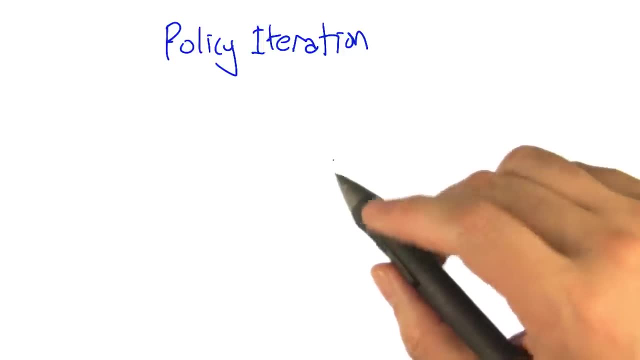 Oh sorry, no, no, no, it's the Ron Howard, the algorithm designer. Oh, that one. I always get them confused. One one played OPI and the other one proved contraction mappings. They're very similar things. 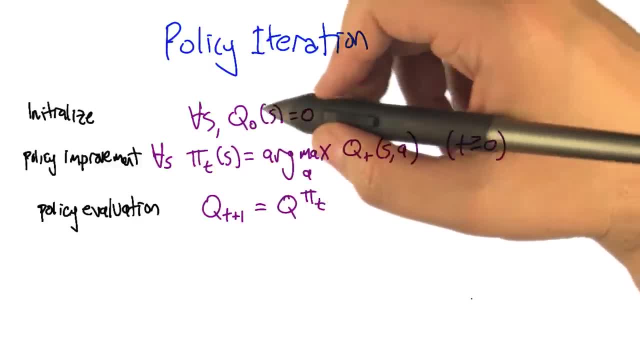 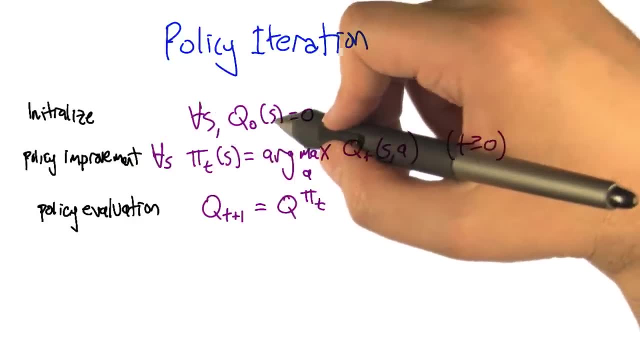 So this is what I was imagining you were explaining Here. let's take it step by step. So what we're going to do is we're going to start off picking an arbitrary Q function, like we often do. We'll call that the initialization step. 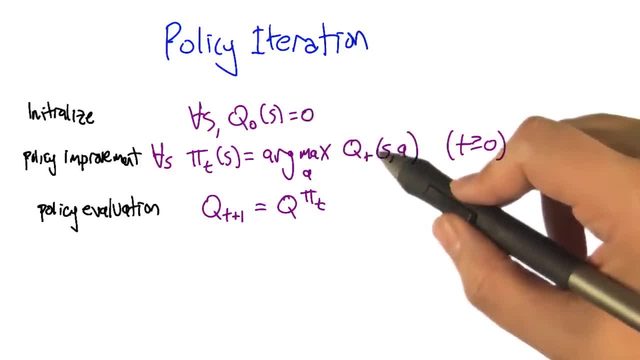 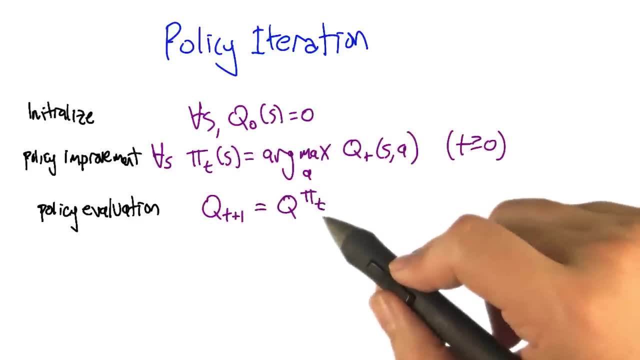 Then we're going to iterate the following: We're going to take the teeth Q function and compute its greedy policy. Call that pi sub t. Then that policy, we're going to evaluate it to get a new Q function: Q t plus one. 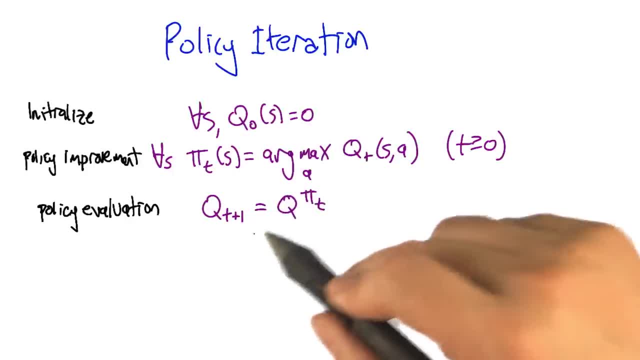 And then we're going to repeat and iterate this over and over and over again. So each time we go around this loop, we're taking our previous Q function, finding its greedy policy, taking that greedy policy, finding its value function and repeating 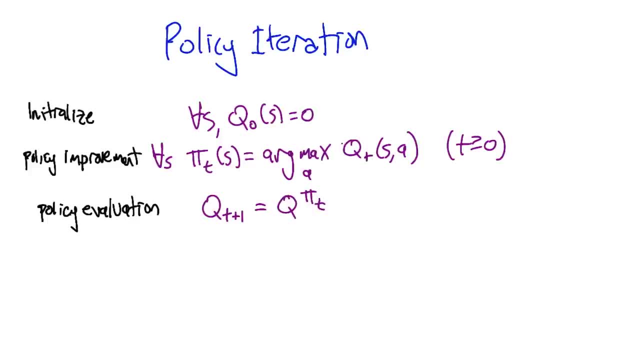 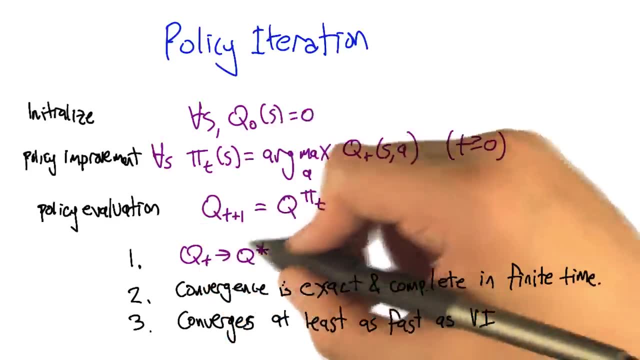 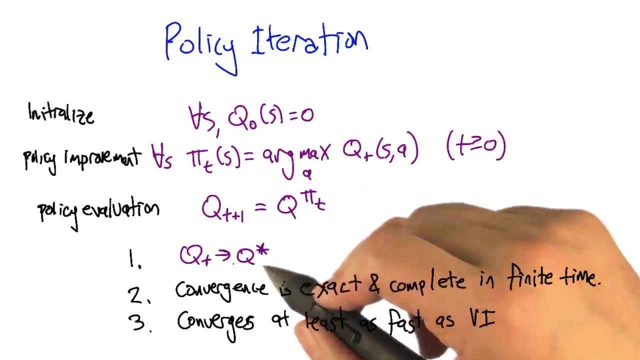 Now the rinse repeat Exactly. So, unlike when I take a shower, we actually get convergence in finite time. So, in particular, the sequence of Q functions that we get converges to Q star, Which is, Which is good. that's like how policy iteration works. 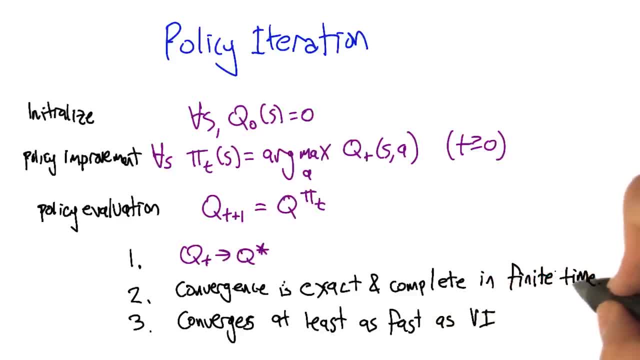 But even better, the convergence is exact and complete in finite time- Though I guess that was kind of true of value iteration as well- And it converges at least as fast as value iteration, in that if at any point we sync up the Q functions, we start value iteration and 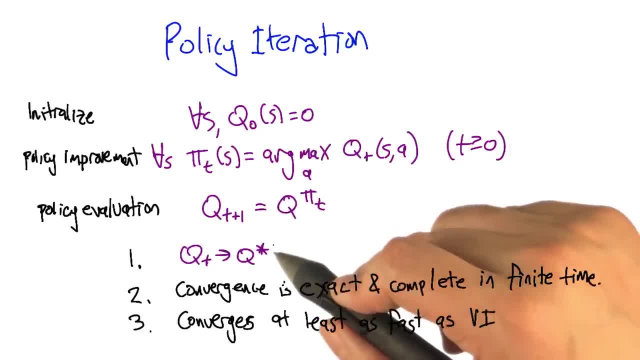 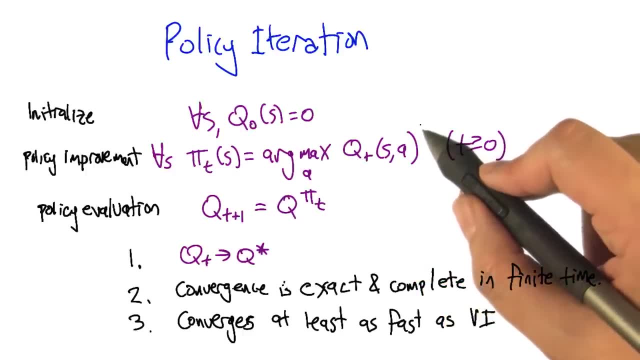 policy iteration from the same Q function, Then each step that policy iteration takes is moving us towards the optimal Q function no more slowly than value iteration does. Okay, So that kind of suggests that this is just way better. Yeah, isn't it way better? 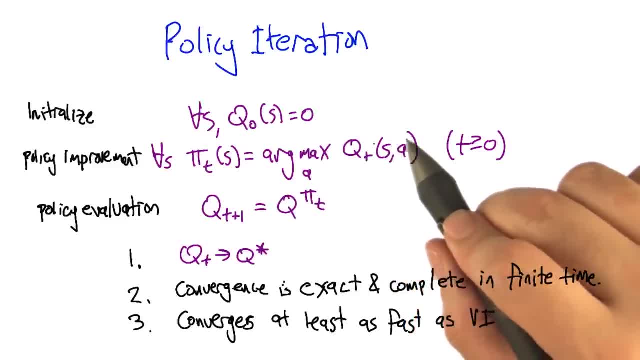 So why is it not way better? There's kind of some excitement going on in here that we need to take into consideration. There is a bit of a trade off, as you like to say, Mm-hm. what's the trade off?